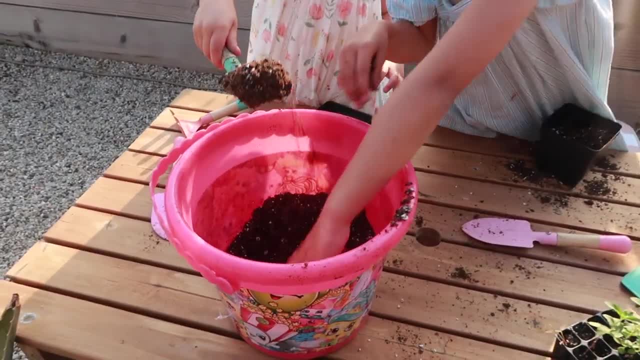 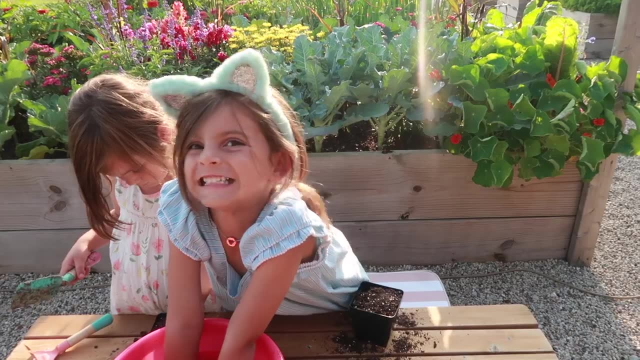 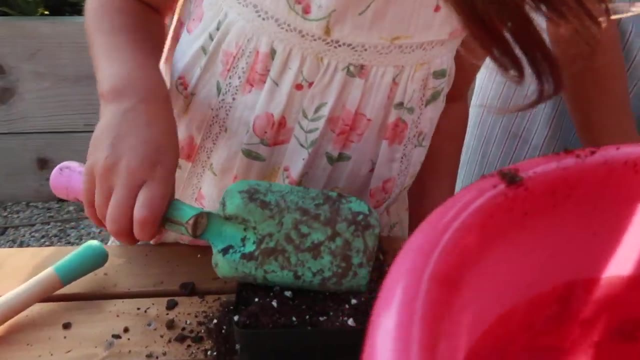 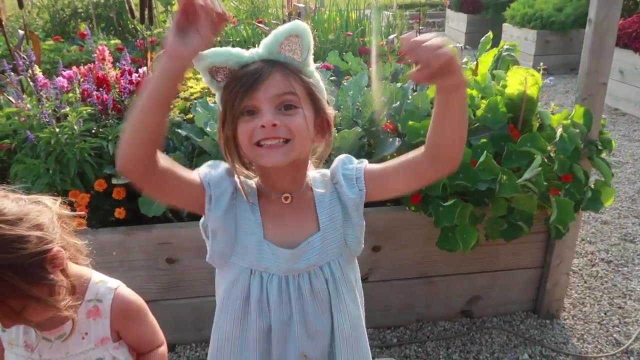 We're using potting soil. It's nice and fluffy and fuzzy, So nice to plant, It's good. You just want to pat some of that off. Pat, pat, pat, Rub it off like this, And it's okay if your hands get dirty. That's all about it Dirty. 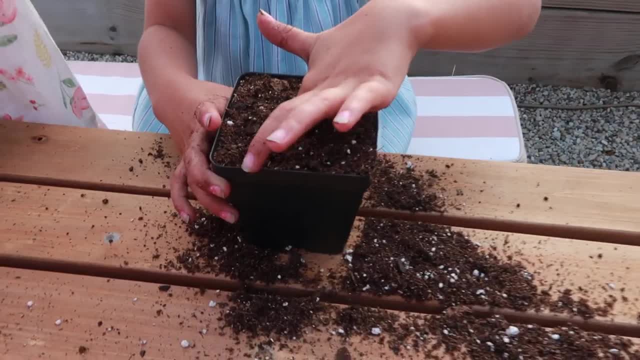 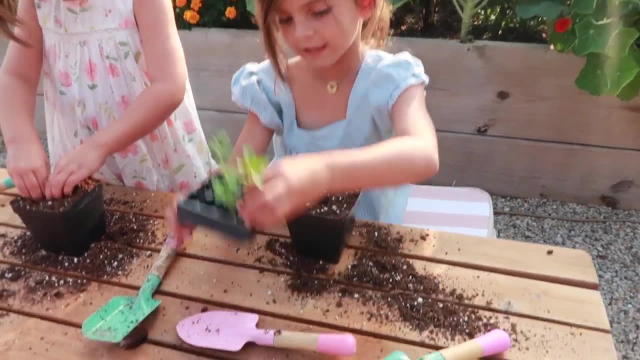 Now it's time to make a hole. You can get it a little deep, but not too deep. Now I'm going to grab the stevia. This is how I take, pull it out. This is how I pull it out. I grab up and I pull it out of the pot. 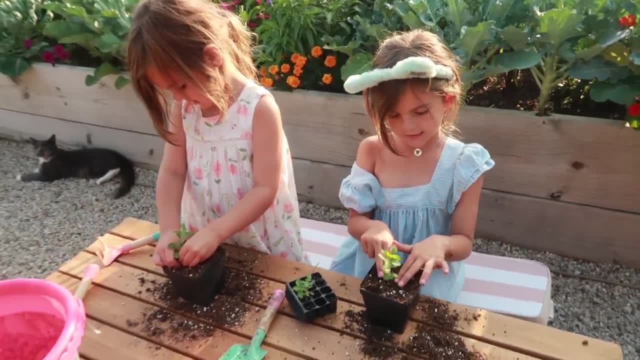 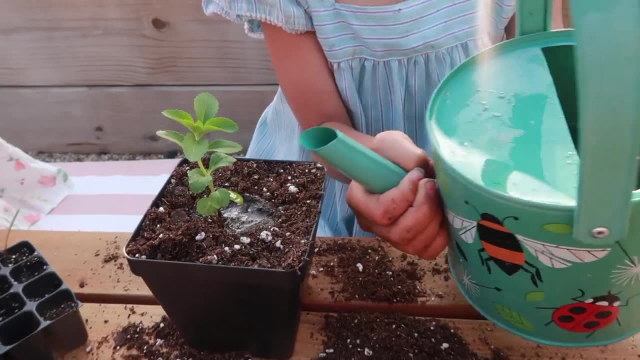 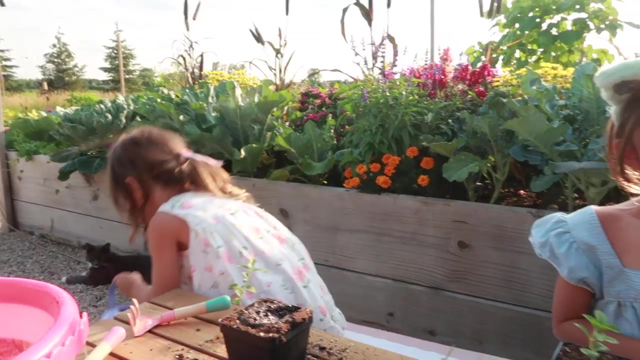 The bottom and then I put it in. I do this And then now it's time to water. Yay, I'm so excited. You don't need a lot, You just need this much. I'm going to pull a leaf off and eat it. It's going to be yummy. 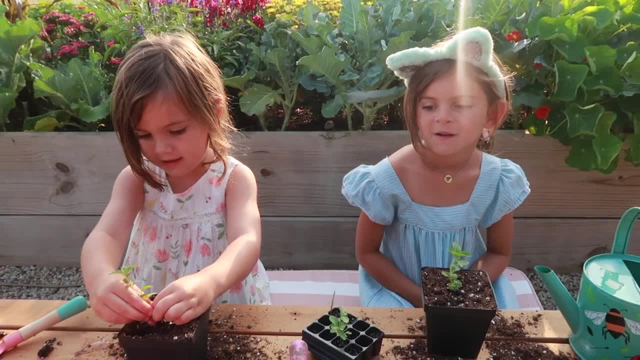 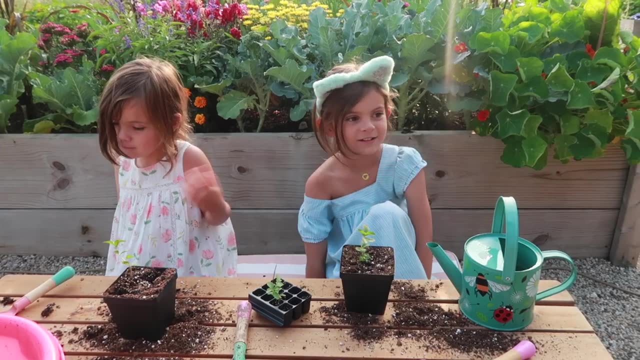 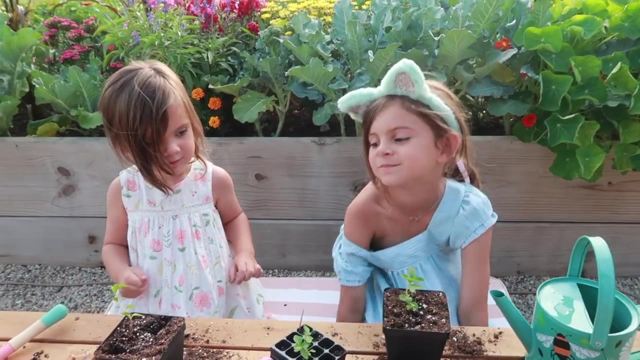 Oh, Oops, One of these. So good, It's sweet. It's really sweet. I like it. It tastes super good. I'm going to eat another one, Me too. You don't want to eat all of it, No. 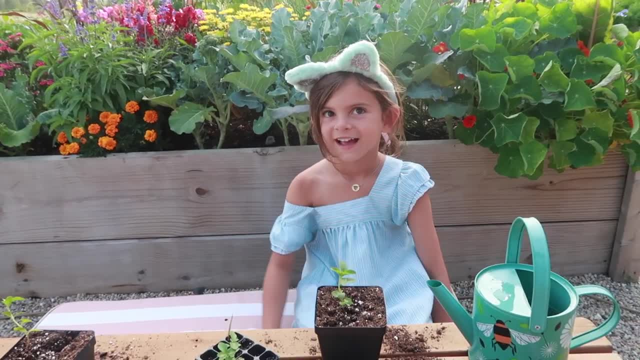 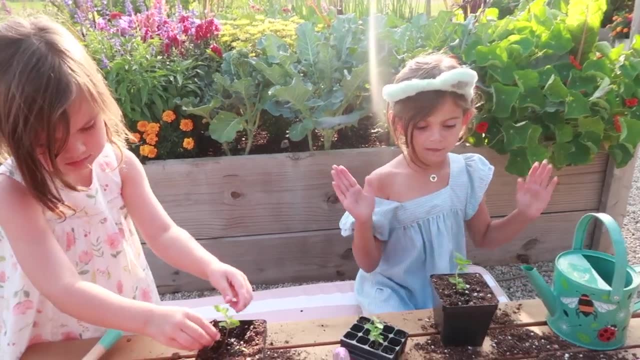 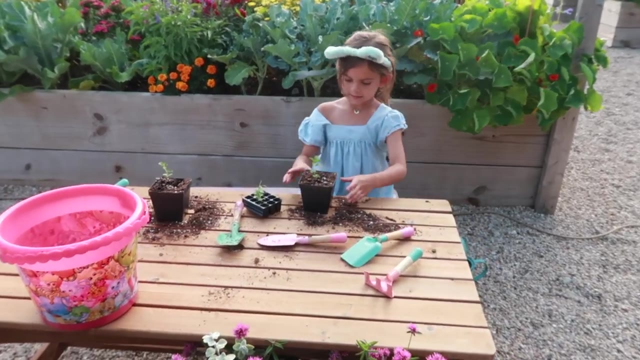 Otherwise you won't have the plant left And you could get gas. It's all healthy. Yeah, Yay, I want to water it again. The next thing is clean up time. First let's put our watering can down, And then we're going to put our plant down. And now let's sweep this off the table. 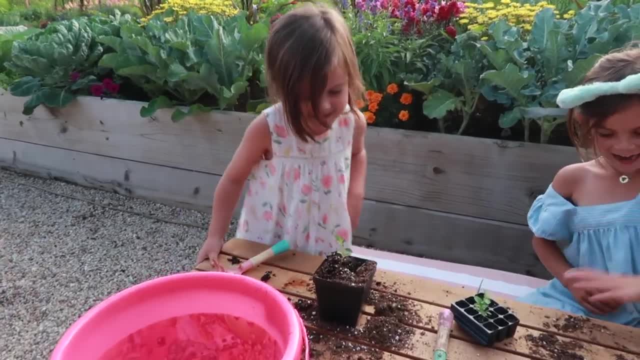 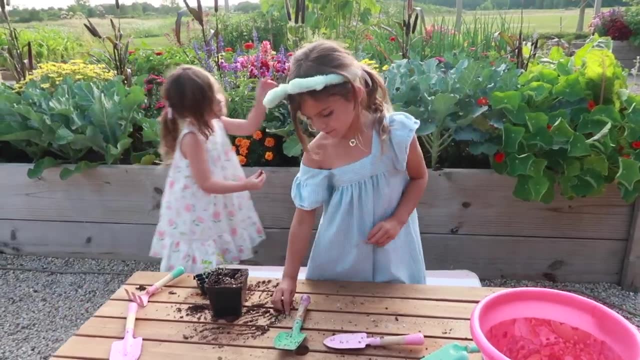 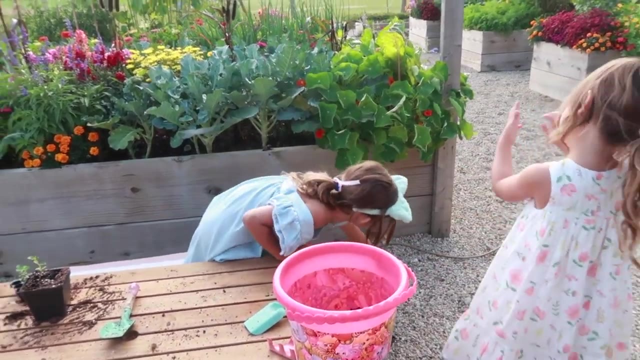 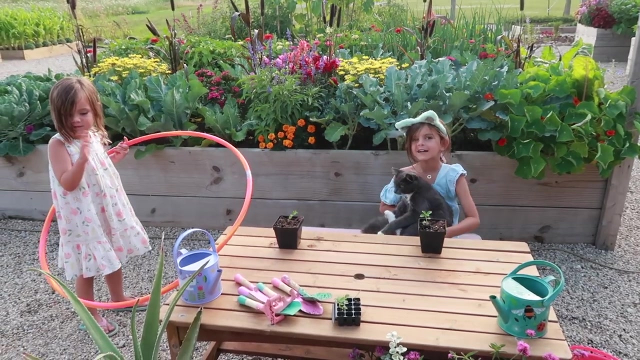 I'm going to kiss the plant. That's amazing. That's giving your plant love. It's clean up time. It's clean up time. It's time to clean up And it's time to end the video. Bye, guys, And remember it's Lana and Selah's Teaching Gardening video.